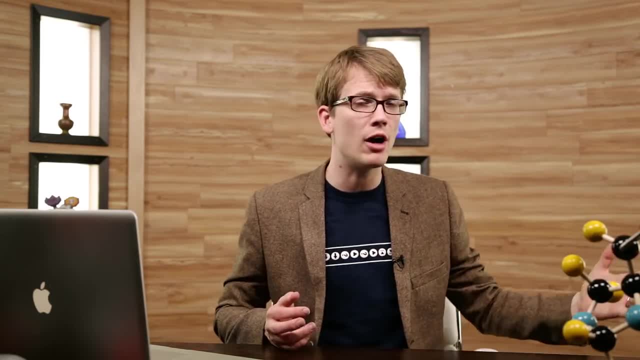 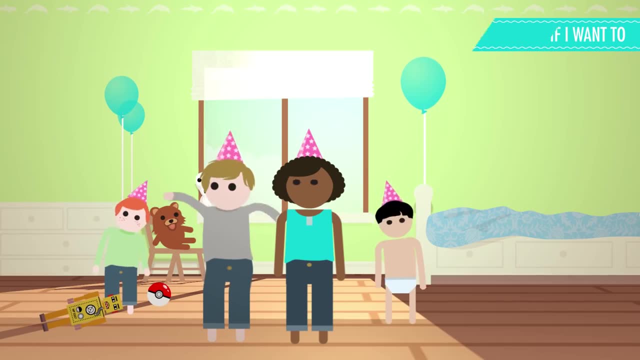 However, as a group they do take up a lot of space. they give off a lot of heat and lots of things get moved around. In these ways, the room is changed by their very presence. Now picture a five-year-old's birthday party. Very different situation, You would not call. 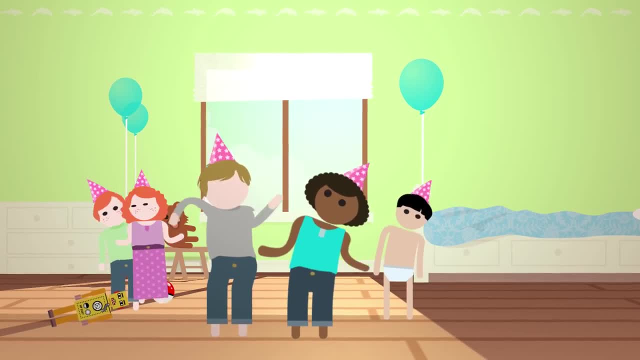 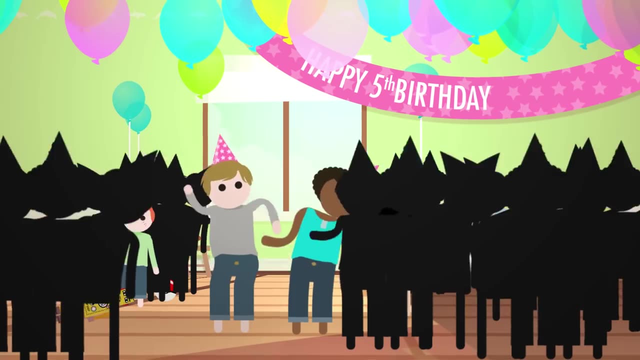 that quiet or formal, But that is not enough. Imagine the most popular five-year-old in the world, his birthday party. Three hundred kindergartners in one room for several hours, shoving each other, running like crazy and definitely banging into walls. Their bodies are smaller, but because of their faster motion they collectively take up just as much of the room and give off just as much heat as the slow-moving adults do, And things get shoved around just as much. Now imagine we have a surprise for those three. 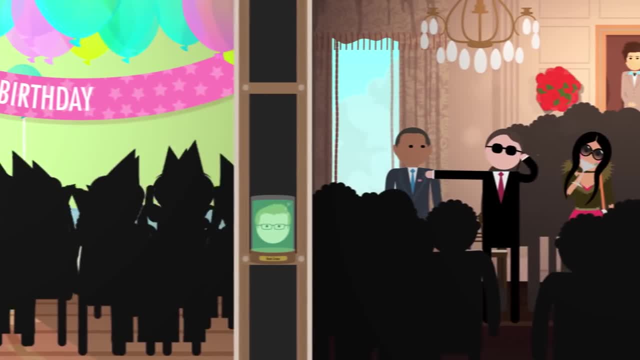 hundred adults at the state dinner, all very formal and tucked in. There are three hundred adults in the room, all very formal and tucked in. There are three hundred adults in the room, all very formal and tucked in. There are three hundred five-year-olds. 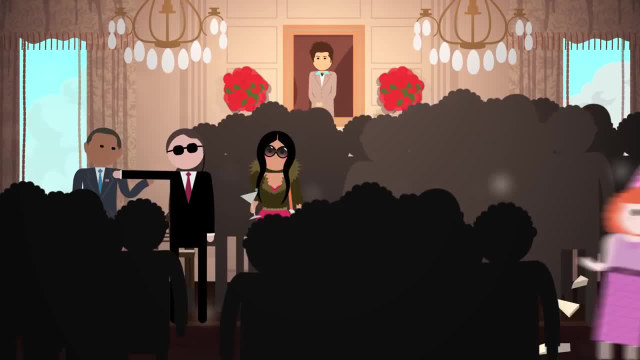 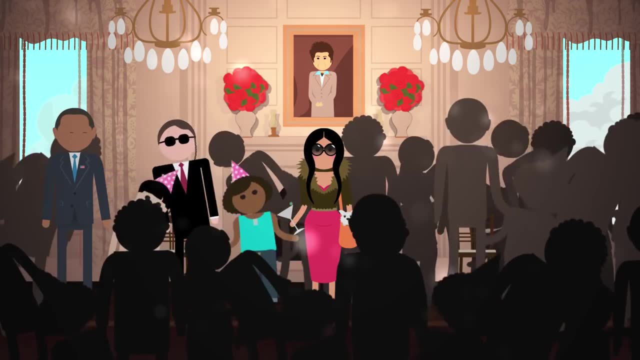 in the next room bouncing off the walls and suddenly we drop the wall. Excellent. First of all, those kids are gonna run all around the room squeezing in between the more sedate adults. That will cause the adults to move apart a little, maybe even bumping. 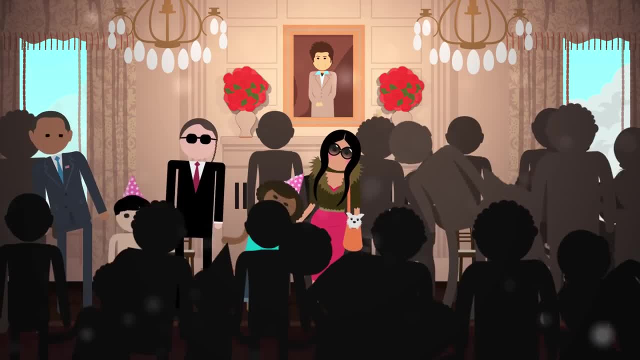 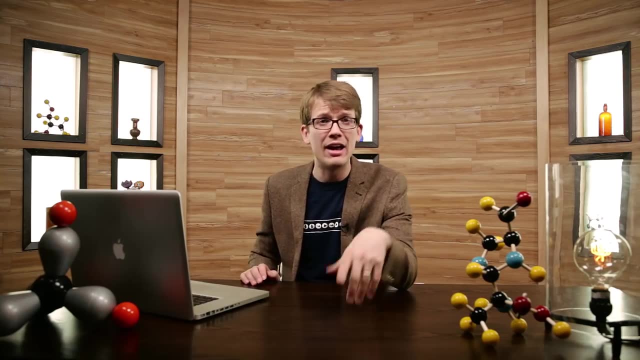 into a wall now and again. But because the adults are moving more slowly they'll get in the way of the kids running and slow them down some. That might even cause the kids to run into the walls a little less often. The most important thing here is that the 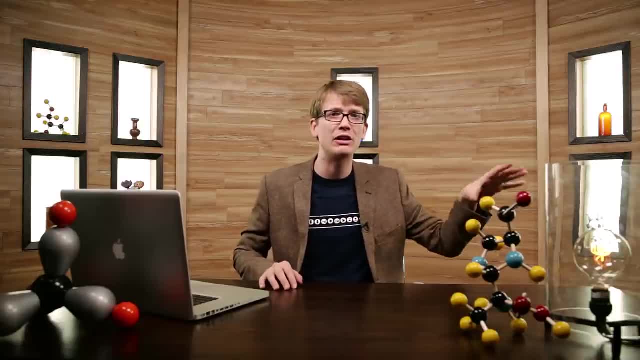 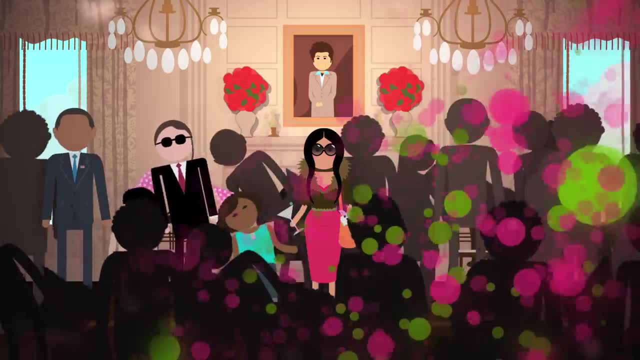 overall bouncing against walls will be equal to the bouncing of the adults plus the bouncing of the kids when they were in separate rooms, And you will not be shocked to find that we are currently in amongst an elaborate analogy to do with gaffes. 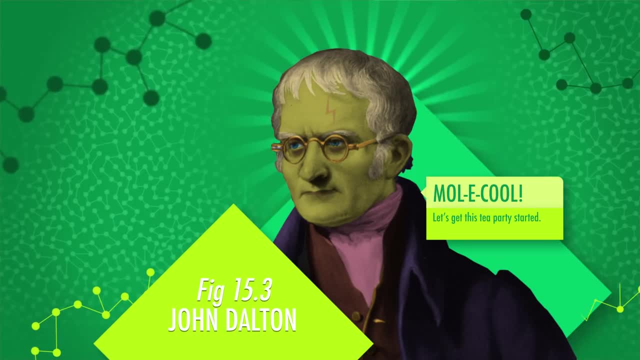 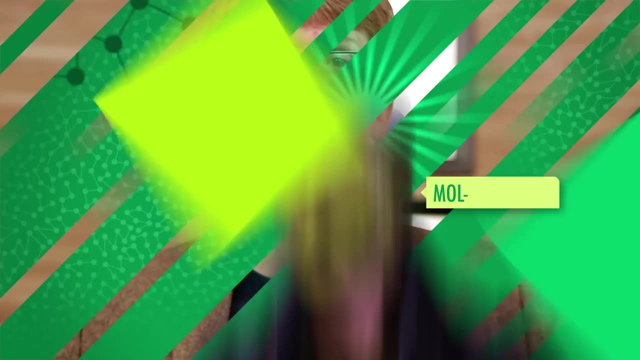 It shouldn't surprise you to learn that this particular party was started by John Dalton, the English teacher, the science teacher from England. He wasn't an English teacher, He was English Who, in 1803, was the first person to use real science to figure out what atoms are and how they behave. 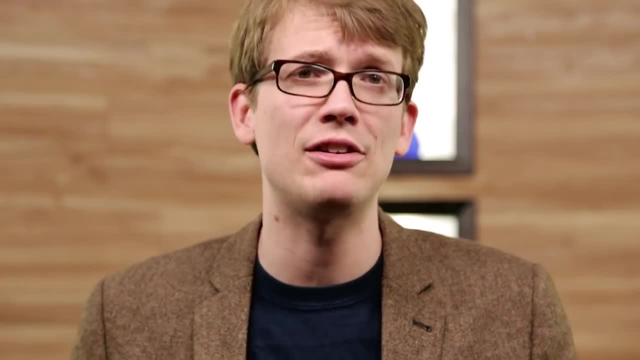 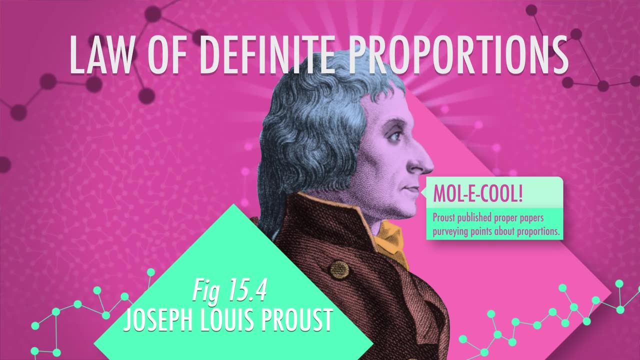 His theory included a few misconceptions, but it contained enough facts to be super useful. Dalton's atomic theorizing began when he expanded French chemist Joseph-Louis Proust's law of definite proportions to develop the law of multiple proportions, which says elements. 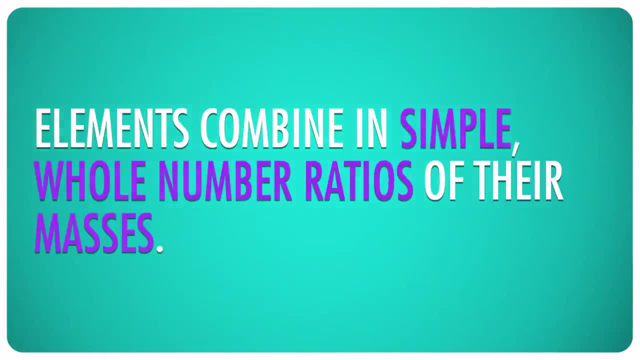 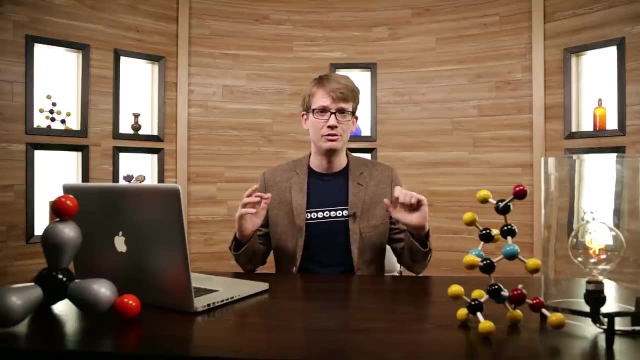 combine in simple whole-number ratios of their masses. But here's the cool part: That exact same research also led to an important gas law. Dalton studied gases basically by mixing them together. He was measuring how much of one element would react with a given 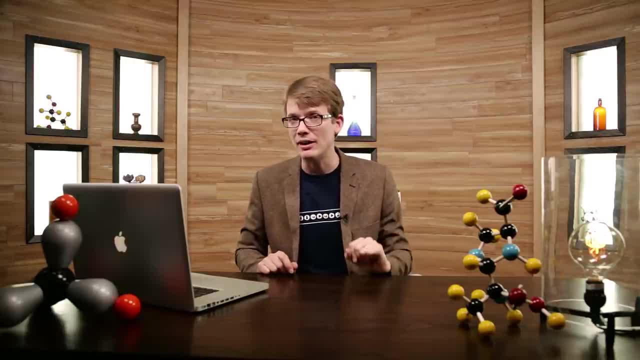 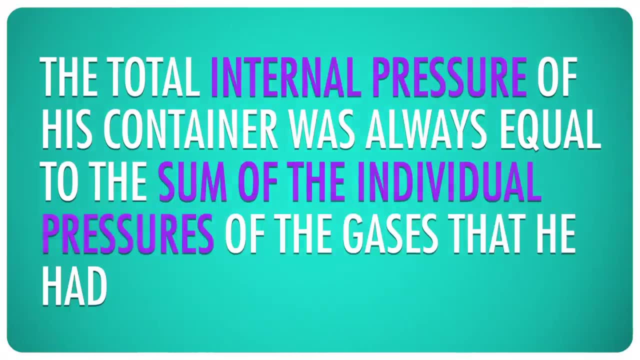 amount of another. But as he mixed those gases, he noticed something else: The total internal pressure of his container was always equal to the sum of the individual pressures of the gases that he had added. Upon recognizing that this happened every single time, no matter. 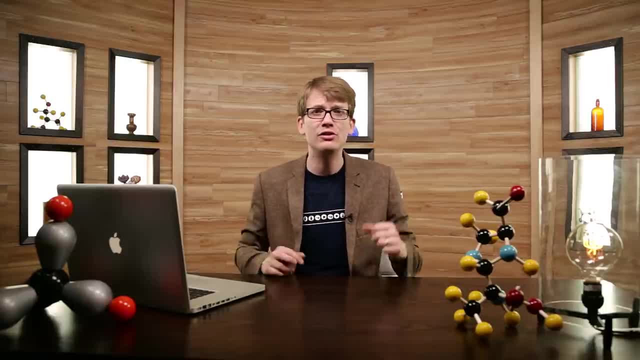 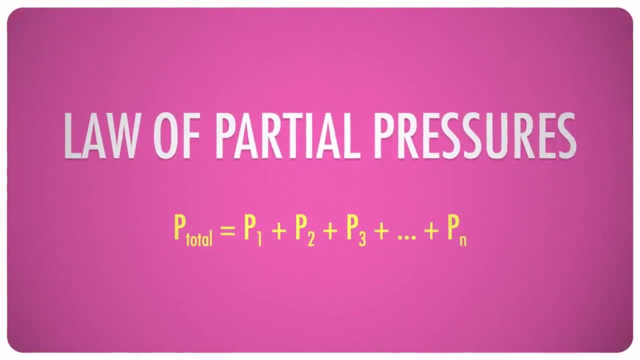 what gases were used or what amounts were added. Dalton stated his discovery as the law of partial pressures. As long as the gases don't react chemically, the total pressure exerted by a mixture of gases is equal to the sum of the individual pressures of the gases that he had added. 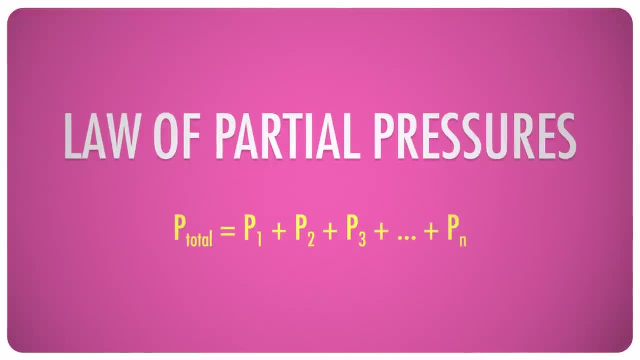 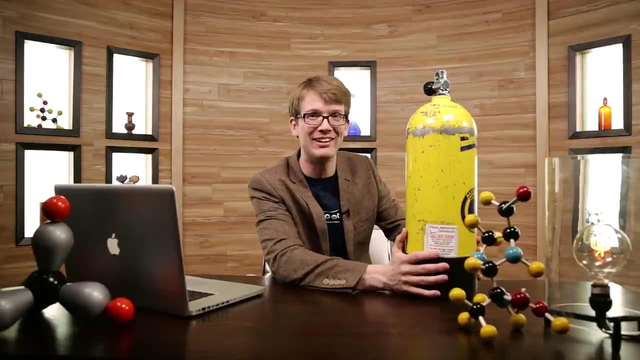 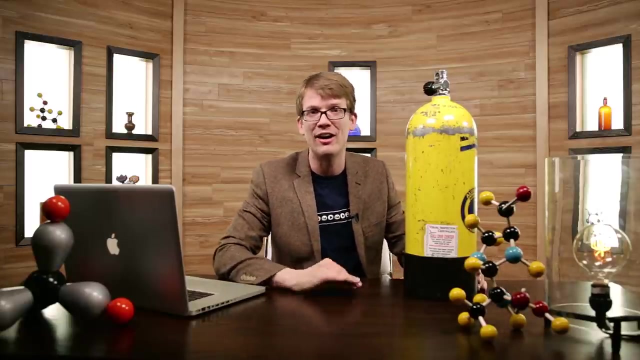 Here's an example: Scuba tanks often contain a mixture of oxygen for breathing, obviously, and helium, which helps prevent decompression sickness because it's released from the blood more readily than nitrogen in air. That allows divers to return to the surface more quickly. 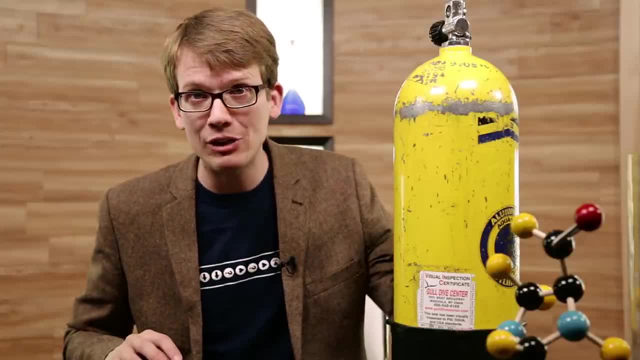 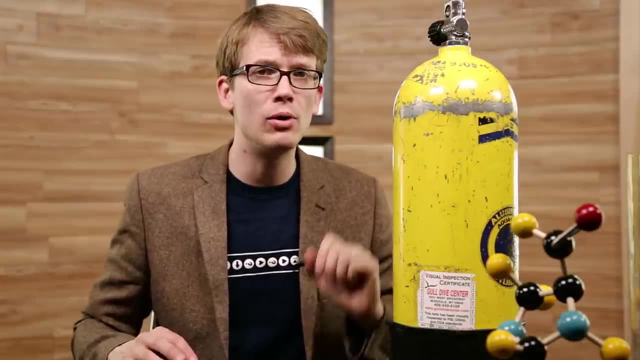 with less risk of gas bubbles forming in their blood. We're gonna use some approximations here, so don't yell at me if you know exactly how big this tank is, but we're gonna say that it's ten liters And we'll say that it contains 4 moles of helium and 1.1 moles of oxygen gas. The temperature: 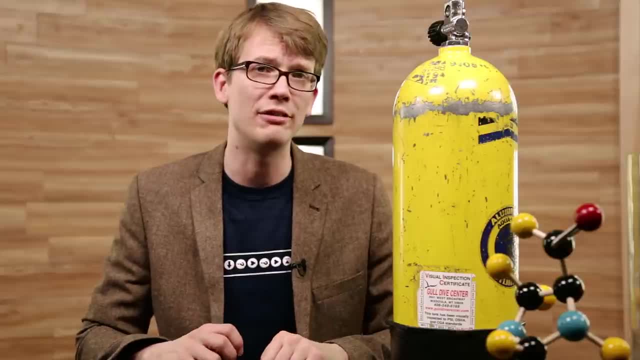 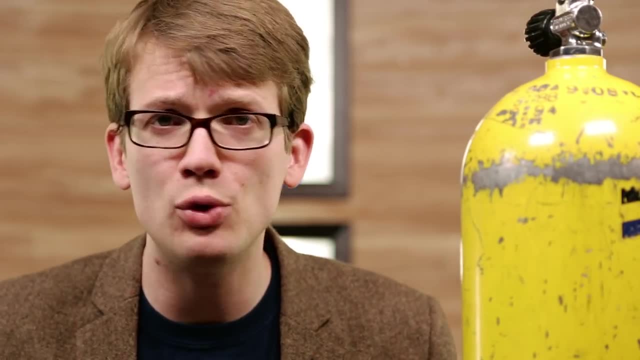 in this room is about 22 degrees Celsius or 295 Kelvin. So what's the total pressure inside the tank? In order to solve that, we need to know the pressure exerted by each gas individually, and we can find that with the ideal gas law. 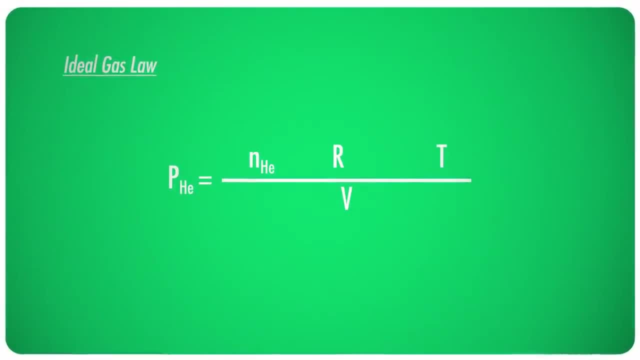 Starting with the helium, we don't know the pressure, so we're solving for P. The volume is 10 liters and we have 4 moles of helium. R is always the same and the temperature is 295 Kelvin. The calculation should show that the helium would have a pressure of 980 kilopascals if. 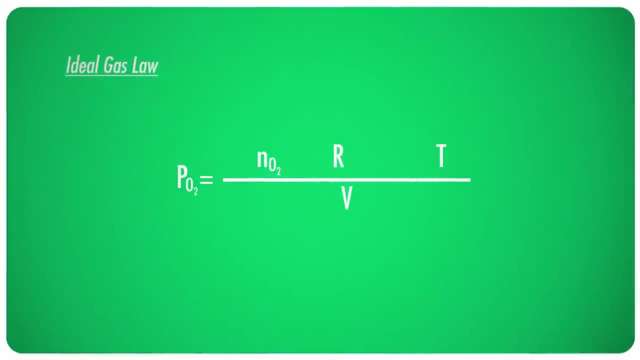 it were alone. Now for the oxygen, all the numbers are the same, except for the moles, which is 1.1 for the oxygen. According to the calculation, the oxygen alone would have a pressure of 270 kilopascals. 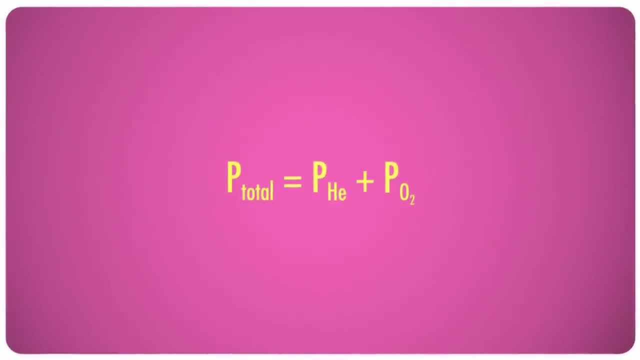 The Law of Partial Pressure says that the total pressure is equal to the sum of the individual pressures. so in this case, 980 plus 270 equals 1,250 kilopascals, or 1.25 megapascals. Easy, isn't it? 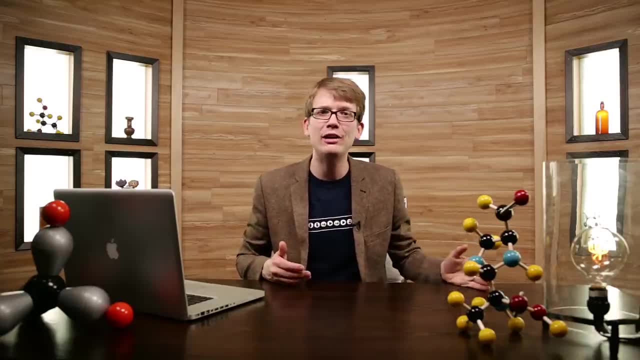 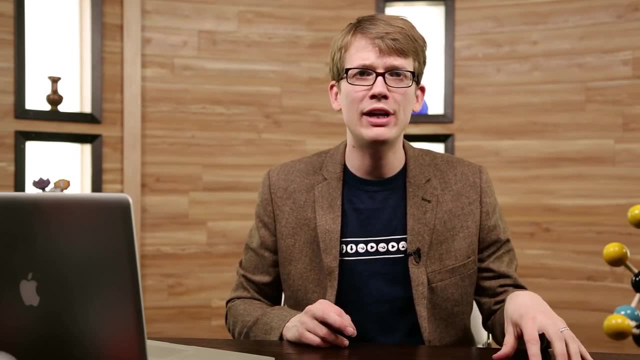 This additive property of pressures is closely related to the fact that mixing gases combines their particles, thus increasing the total moles of gas present. The ratio of moles of the individual gases in a mixture to the total number of moles is called the mole fraction. And of course, mole fraction gets to have its own little esoteric symbol to represent it, the lowercase Greek letter chi, Chi sub one. the mole fraction of an individual gas equals N sub one: the number of moles of that gas divided by N sub total: the total number of moles in the mixture. 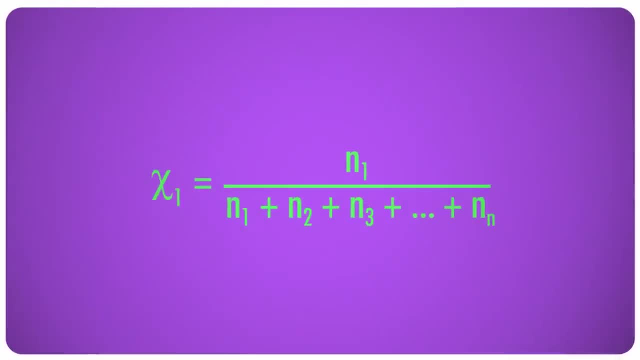 And because the total number of moles is the sum of the moles of all the gases, we can also say that chi sub one equals the moles of any one gas divided by the sum of the moles of all the individual gases. You see how that last formula looks a lot like the one for partial pressures. That's because they're basically the same thing. Through the ideal gas law, the number of moles is directly related to the pressure a gas exerts, as long as the volume and temperature remain the same. So you may have figured this out already, rather than having to calculate individual. 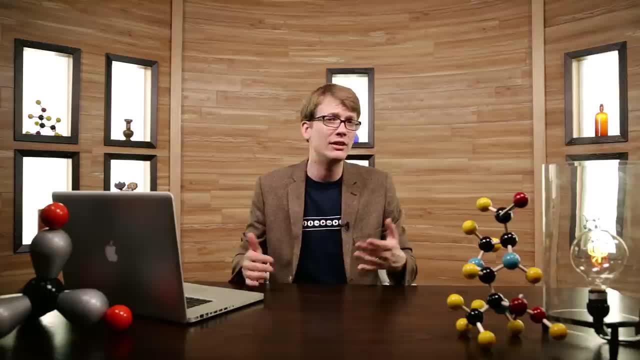 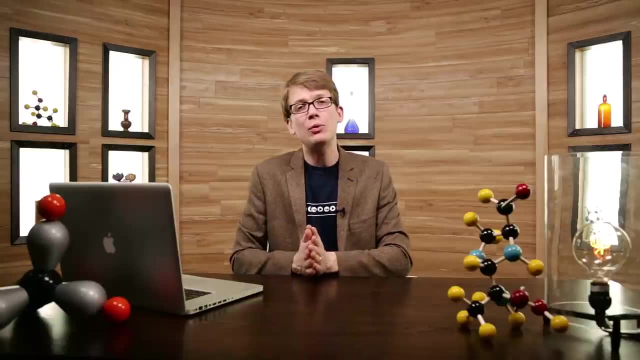 pressures first every time, as we did with the scuba tank, or calculate the individual moles. in the opposite situation, we can often calculate what we need directly from what we already know. Let's give it a try. The air that we breathe is about 21% oxygen, or 21 parts oxygen in 100 parts air. 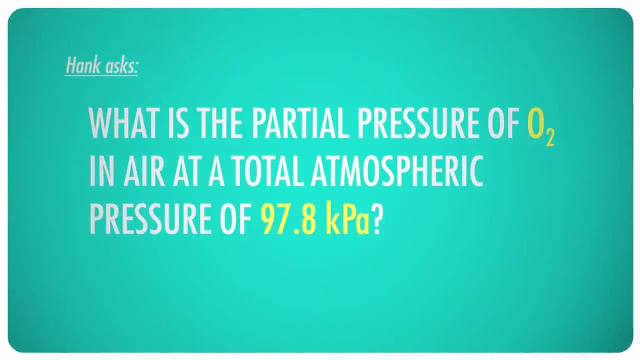 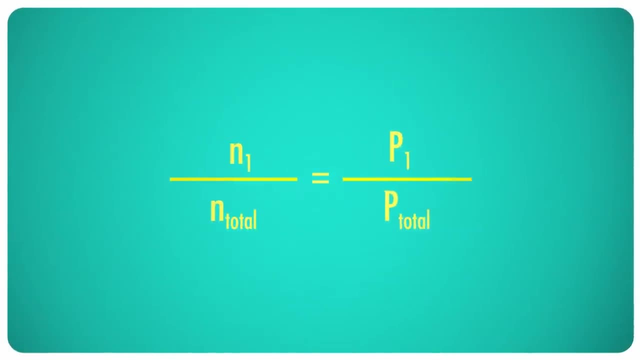 What is the partial pressure of O2 in the air at a total atmospheric pressure of 97.8 kilopascals? We can substitute moles for parts and use the mole fraction formula. Plug in 21 moles of oxygen for the individual gas and 100 moles of air for the total amount. 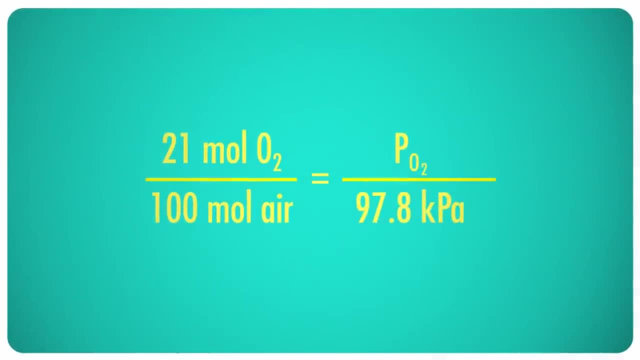 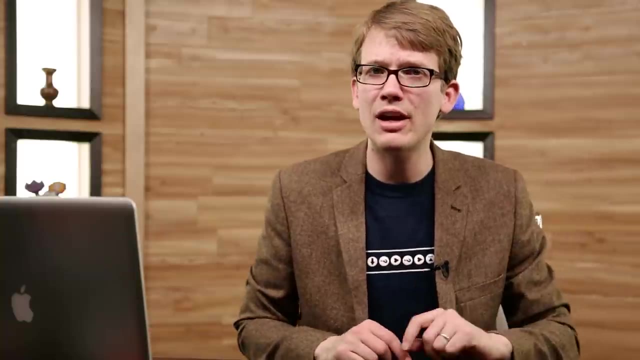 then put in the total atmospheric pressure, 97.8 kilopascals, and do the equation. With correct rounding, that'll give you a partial pressure of 21 kilopascals for oxygen. Sometimes, however, gas is mixed together in ways that aren't so predictable. 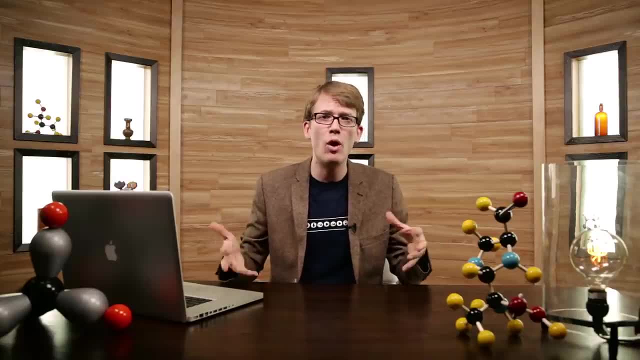 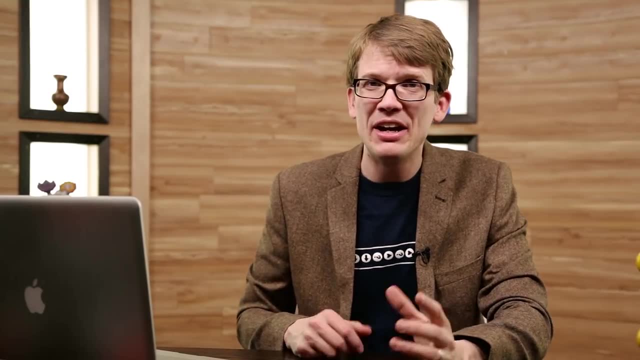 For instance, one way to collect a gas is by bubbling it through a column of water to trap the gas at the end of the column. This is called collecting a gas over water. The only problem is that liquid water constantly is giving off a small amount of water vapor. 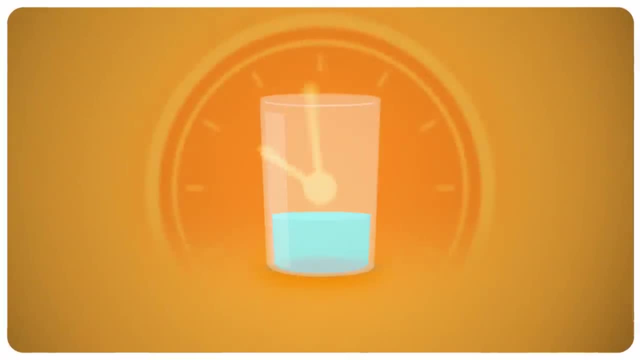 That's why, if you leave a glass on a desk for long enough, there will eventually be no water in it. There are always going to be a few molecules that have enough kinetic energy to escape the liquid. The amount of vapor that's released depends on the temperature of the water. 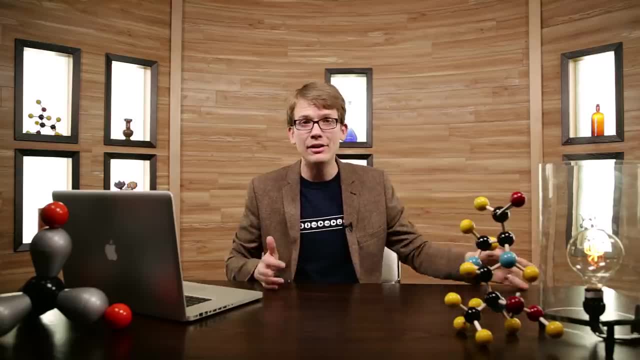 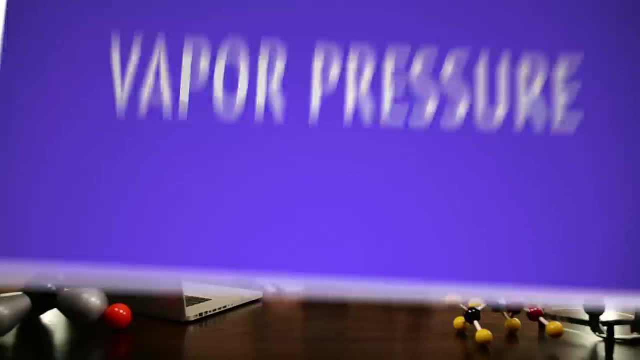 The more heat energy it has, the more vapor we get. Like all gases, the water molecules move around a lot and sometimes bump into the sides of the container, thus creating pressure. This is called the water's vapor pressure. The water molecules move around a lot and sometimes bump into the sides of the container. 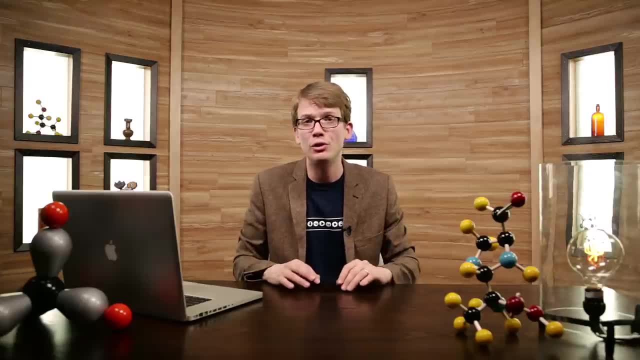 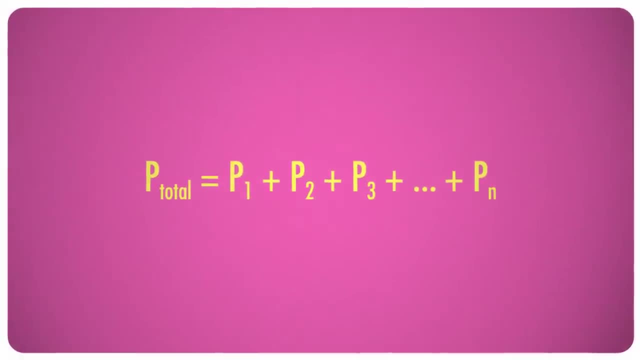 thus creating pressure. The water molecules mix with the gas that's being collected, and when that happens, as good old John Dalton taught us, total pressure in the column equals the pressure of the collected gas plus the vapor pressure of the water. So to know how much gas we really collected, we have to subtract the vapor pressure of 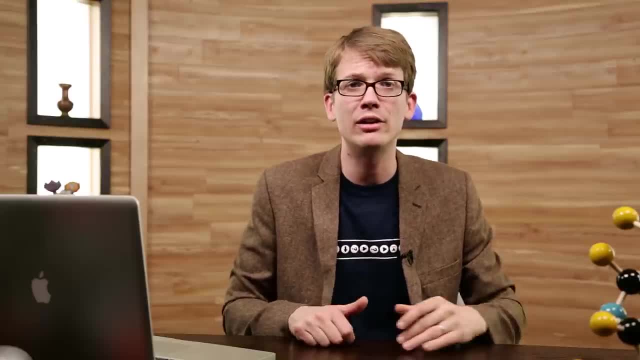 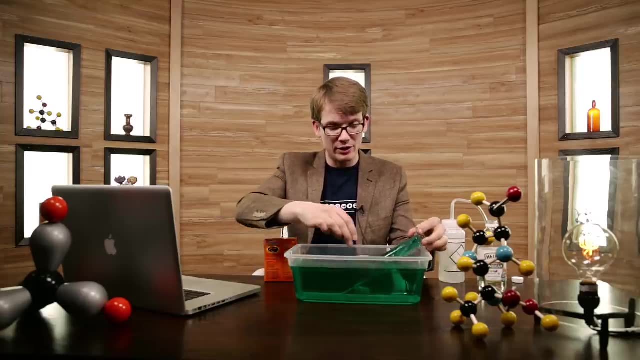 the water from the total pressure. This gives us the pressure exerted by the collected gas, and from that we can calculate the moles of gas present. Here's how it's done. Here I have a tub of water and a graduated cylinder that I've put into the water and 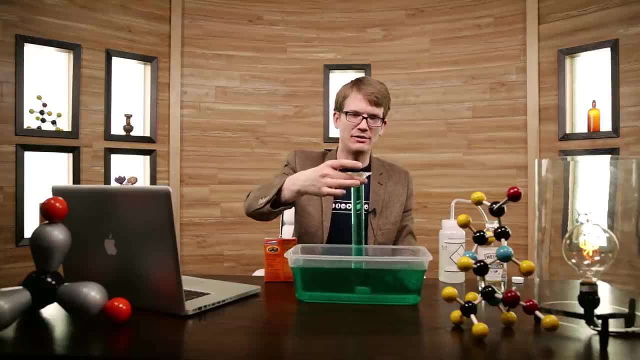 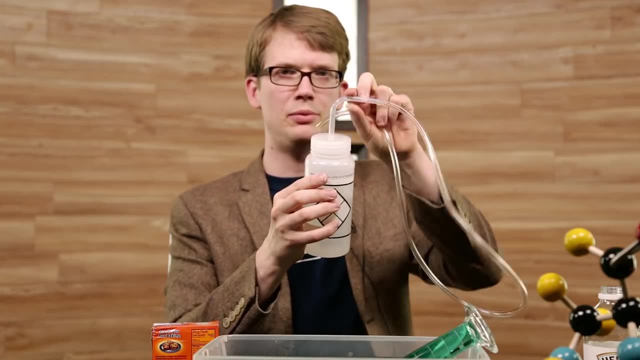 then filled with water. So now you can see it's got no gas in it, just water, And we are going to capture gas in here and see how much gas we capture Here. I have a bottle and it's sealed with this little tube. 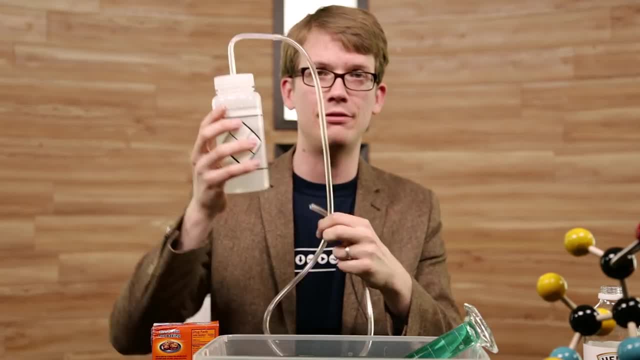 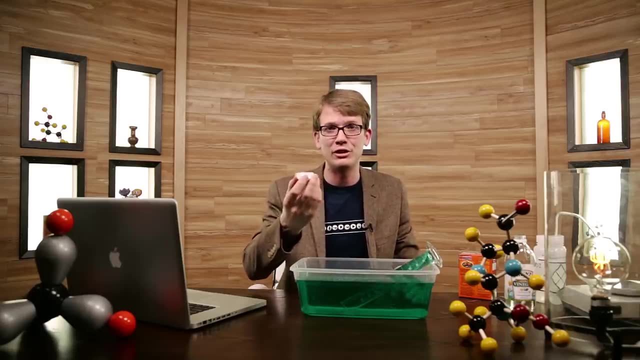 This is the only way for gas to get out of here And in here right now I have vinegar, an aqueous solution of acetic acid. This is baking soda, more properly, sodium hydrogen carbonate or sodium bicarbonate. I think we all know what will happen when this comes in contact with vinegar. 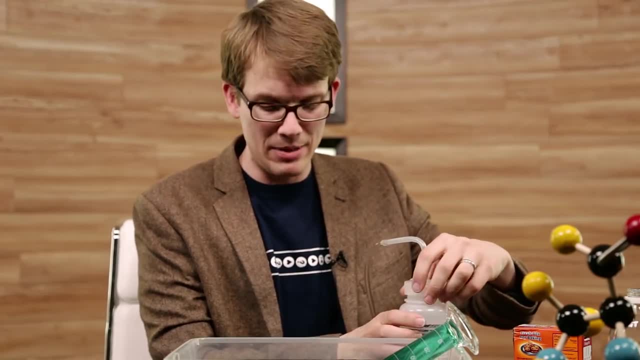 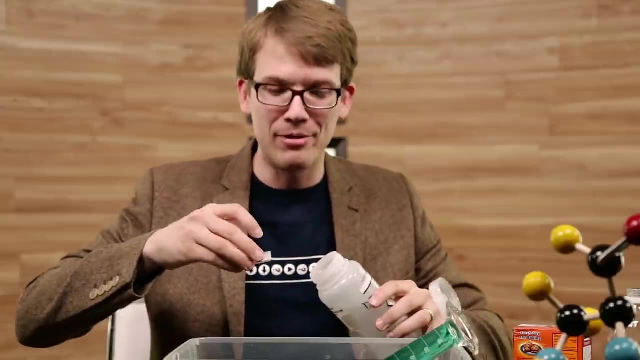 Now, to prevent that from happening before I won't- This isn't happening before I want it to happen. I made it a little boat for it, And the boat is theoretically, I hope, going to sit on top of the level of the vinegar. 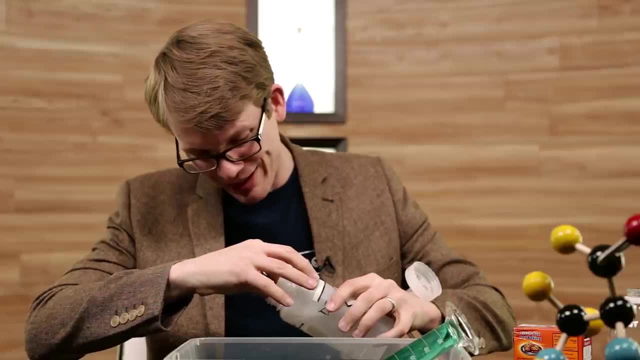 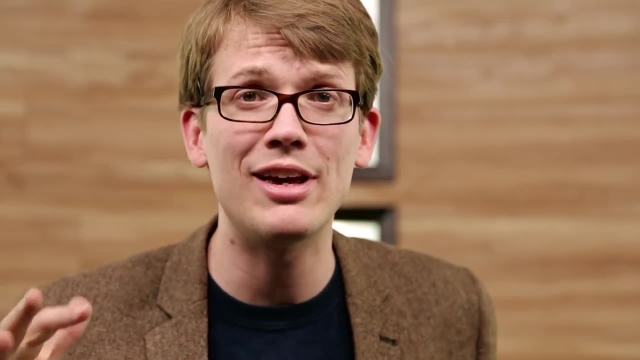 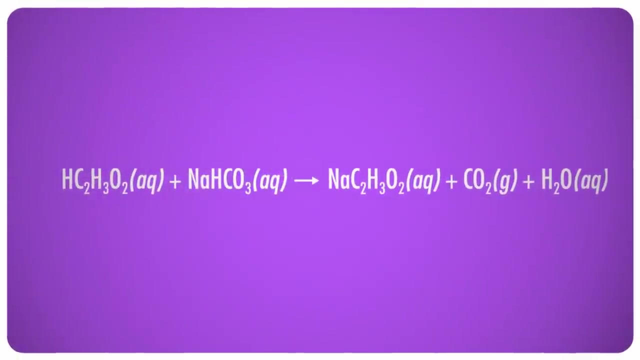 and float there without spilling. Yeah, yeah, yeah, I did it. Before the big action scene, let's talk about what's actually happening chemically speaking, because, as you know, I love to speak chemically. The acetic acid and sodium bicarbonate combine. 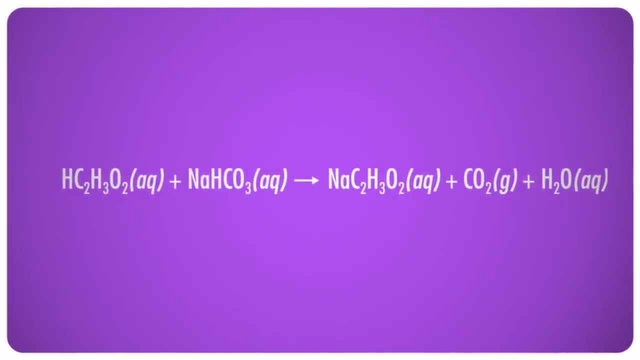 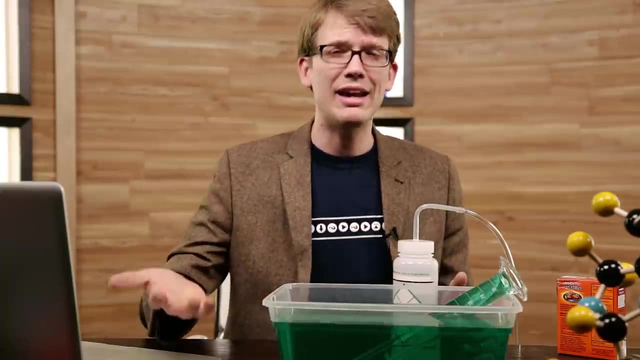 They form sodium acetate, carbon dioxide and water. The sodium acetate dissolves readily in water and will stay that way. The carbon dioxide, on the other hand, is the source of all our fun. It's a gas and it forms so many little bubbles in the surrounding liquid that it's almost 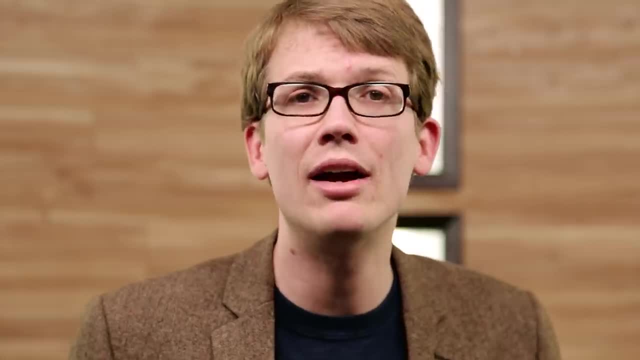 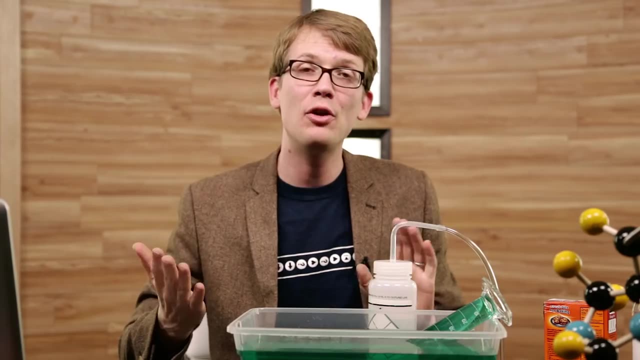 a foam expanding quickly and dramatically. As the carbon dioxide escapes through the foam, it goes through the tubing and bubbles through the column of water. so we get double the bubbles, double the fun. And don't forget, at the end we'll be able to calculate how many moles of CO2 are produced. 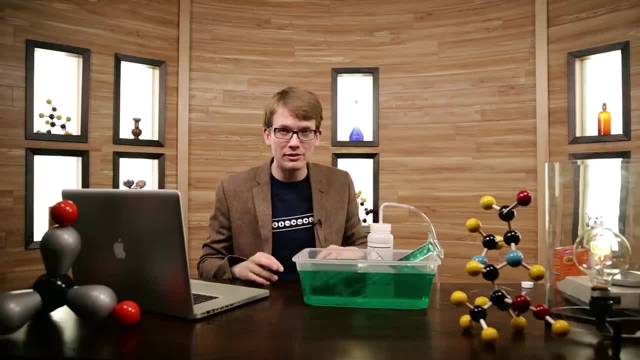 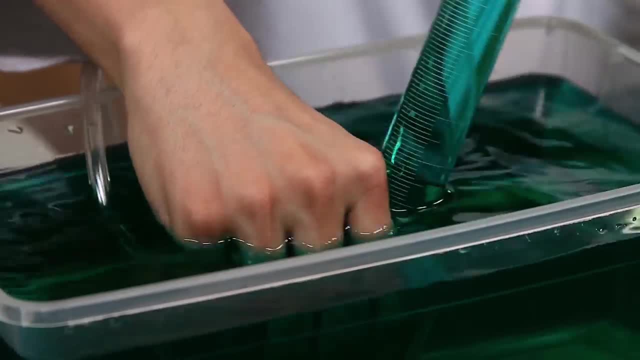 by this reaction. Let's get to it. It's going to take more than two hands to do this, so I have a lab assistant with me here today. This is Michael Aranda. All right, Michael, put the tube into the cylinder there and I get to do the fun part. 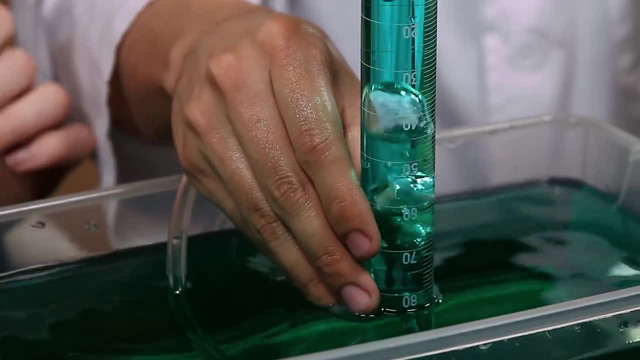 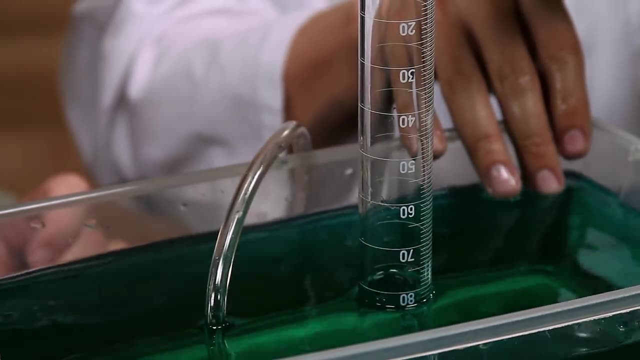 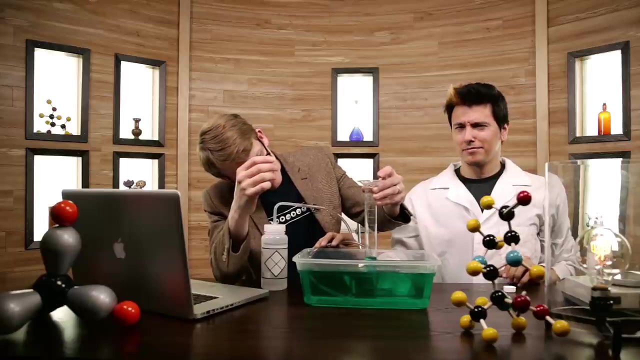 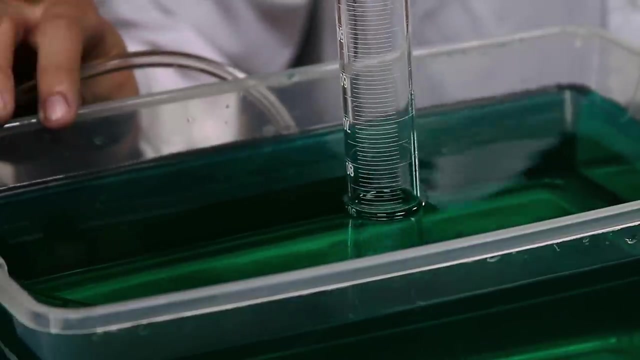 which is to shake this and make bubbles. Bubbles A little more, a little more, a little more. So we have collected exactly about 90 moles of CO2.. Nine, almost exactly 90 milliliters, So like 90.5 milliliters of carbon dioxide. 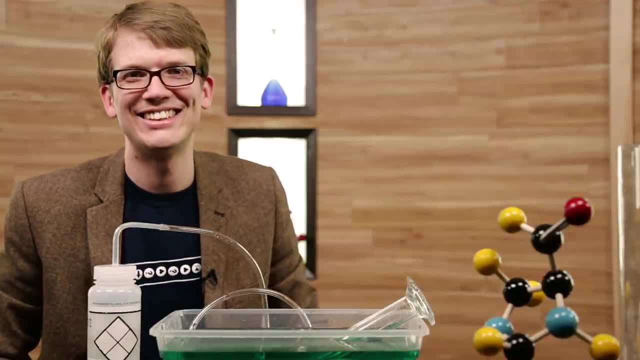 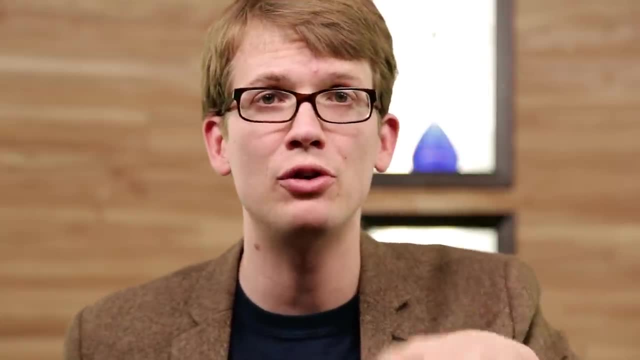 You can go away now. We also know, because I know, that the atmospheric pressure is 101.8 kilopascals- remember, we also need to know what the vapor pressure of the water was that we have to subtract. The amount of vapor pressure that water gives off depends on its temperature, and there's 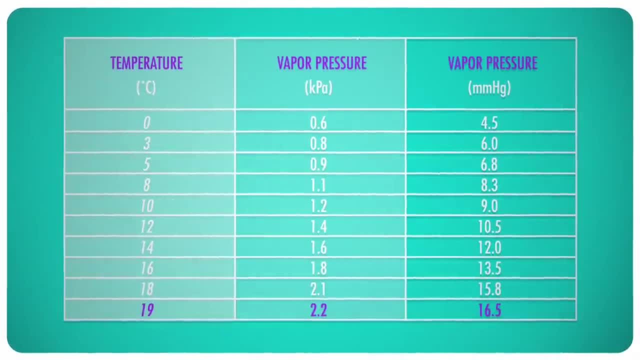 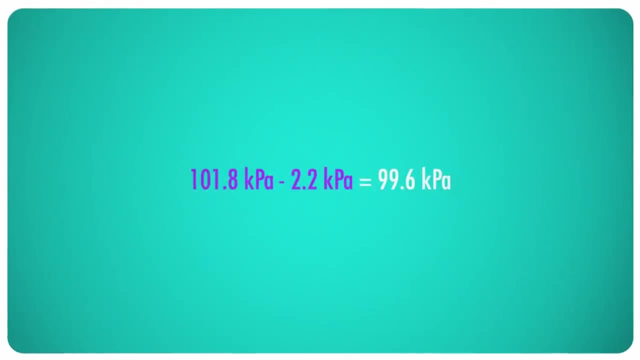 a table we can look at, and if the water is at 19 degrees Celsius, according to the table, the vapor pressure is 2.2 kilopascals. So now finding the pressure of the carbon dioxide alone is easy. We simply subtract 2.2 kilopascals from 101.8 to give us a pressure of 99.6 kilopascals. 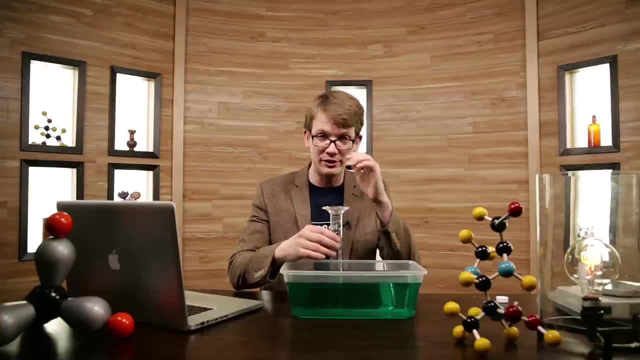 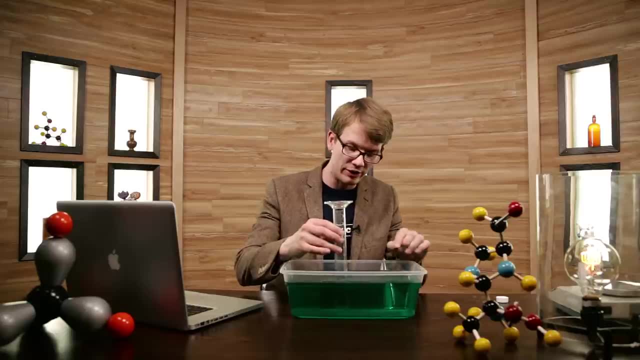 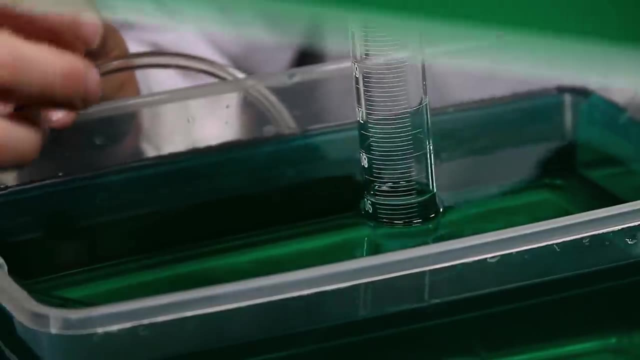 for the carbon dioxide. Finally, we have to make sure that the pressure inside the graduated cylinder is the same as the atmospheric pressure, and to do that, we just have to make sure that the levels of both of the liquids are the same, And doing that, I can see that it is almost exactly 90 milliliters of carbon dioxide in. 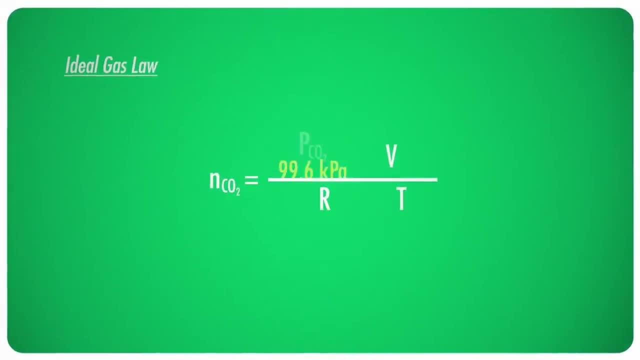 the cylinder. And now we plug everything into the ideal gas law: P is 99.6 kilopascals, V is 0.09 liters, N is what we're trying to find, R is always the same and the temperature is 292 Kelvin. 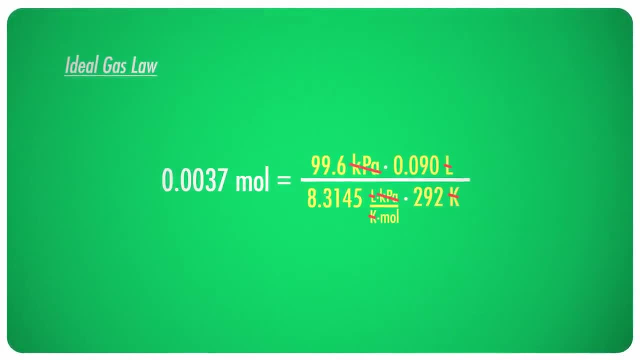 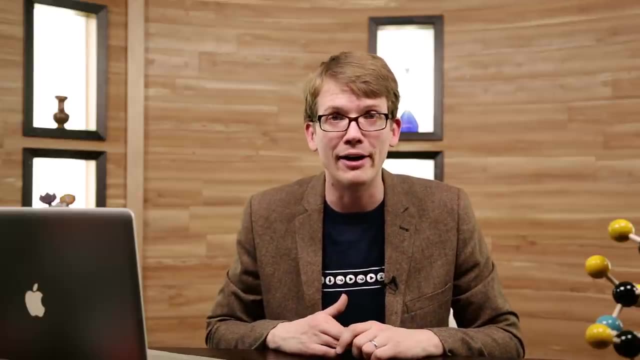 One quick calculation and we find that we have collected 0.0037 moles of CO2.. At a molar mass of 44 grams per mole, that's 0.16 grams of carbon dioxide. I am excited by our success here. 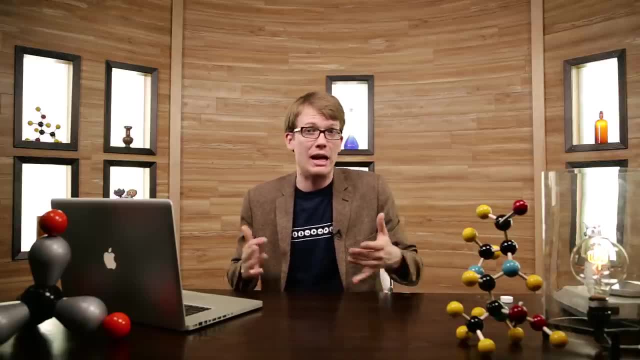 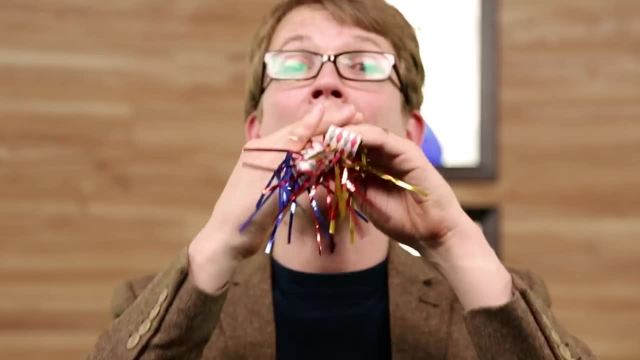 That might not sound like a lot, but collecting a fairly substantial amount of carbon dioxide, a substantial amount of gases, and being able to make accurate measurements of them with a simple apparatus like that is pretty impressive. For me, it sounds like time for a party. 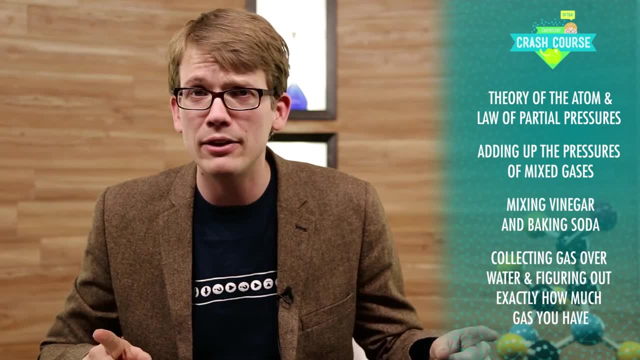 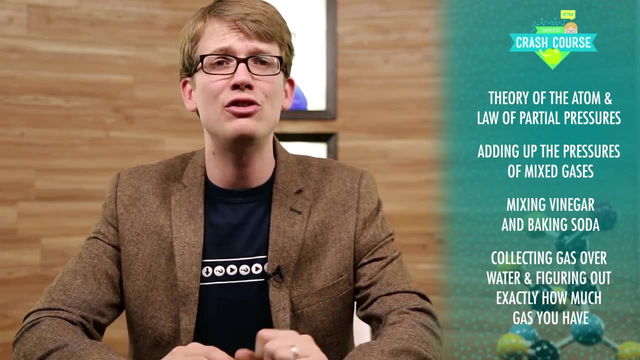 Thank you for watching this episode of Crash Course Chemistry. If you weren't late to the party, you learned that John Dalton built both his theory of the atom and his law of partial pressures on the foundation laid by Joseph-Louis Proust, And that you can add up the pressures of mixed gases just as you can do with their amounts.